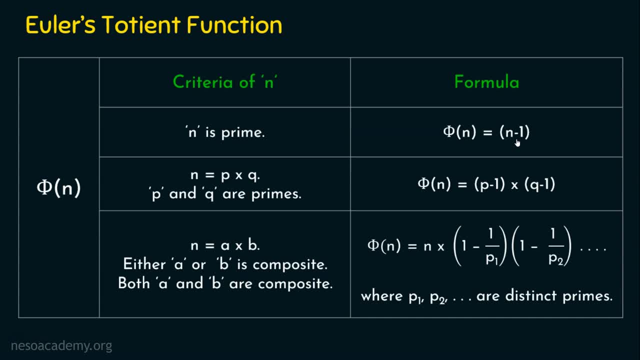 that are less than 7 are relatively prime to 7.. That is what the Euler's torsion function is all about. So this is what the first criteria when n is a prime number, That is this n. If this n is not a prime number but it is a product of two different prime numbers, 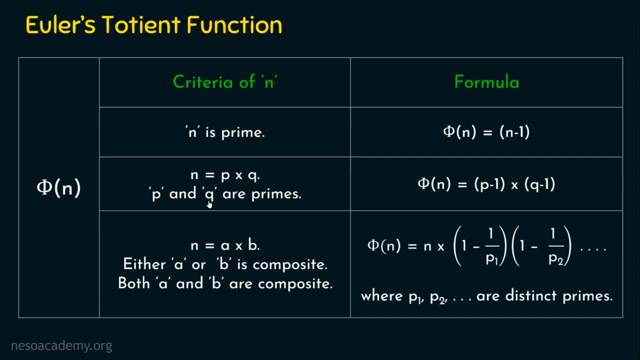 say p and q, For example 21.. So 21 can be a product of two different prime numbers, 3 and 7, right? So in such case you need not manually calculate phi of 21. rather you can apply this formula: phi of n is: 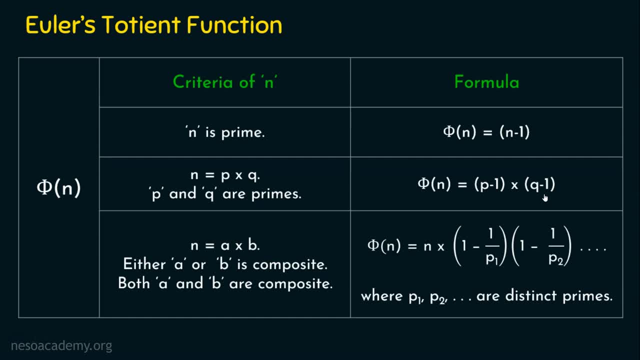 equal to p minus 1 into q minus 1.. In the example we have taken 3 into 7, right, because we have taken 21.. So 21 can be 3 into 7.. So the answer for phi of n can be if p is 3.. So which is 3 minus 1 into. 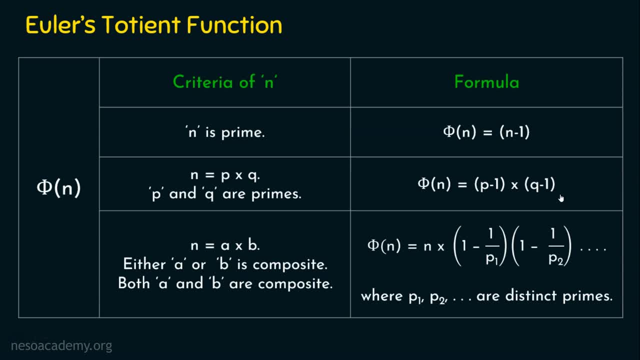 7 minus 1.. In other words, 2 into 6, 12 right. So phi of 21 is equal to 12.. No worries, Anyway, when you see some examples, you will understand things clearly. Let's see the third scenario, The third. 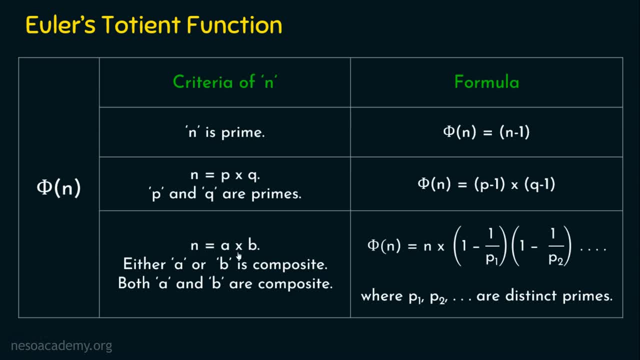 scenario is where we have n, where this n is a product of two different numbers, but these two are not prime numbers. They are composite numbers. In other words, either a is a composite number or b is a composite number, or both a and b are composite numbers. In the previous case, we had a composite number, n, but 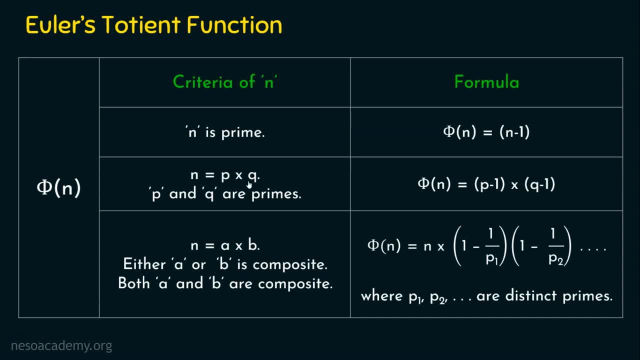 still that composite number is a product of two different prime numbers. There are situations where this n is a composite number, like the previous case, but this n is not a product of two different prime numbers. It is a product of two different composite numbers, or one composite number and 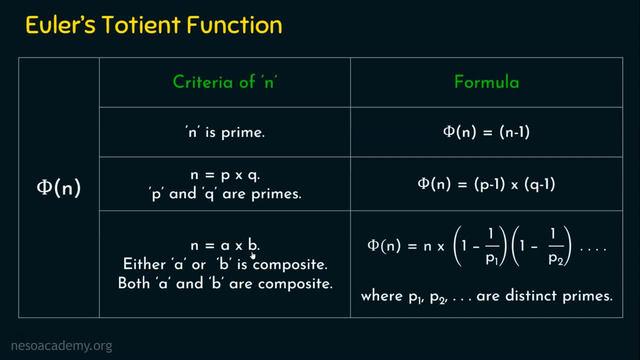 one prime number or both are composite numbers. In such case we need to have some formulas right. So the formula is phi of n is equal to n into 1 minus 1 by p1, into 1 minus 1 by p2, into 1 minus 1 by p3, and you: 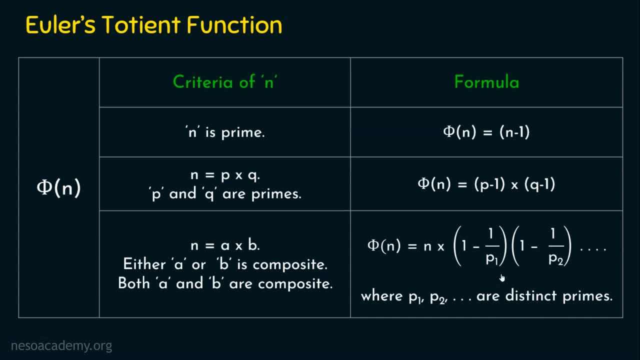 continue this as long as you get the distinct primes Here. p1, p2 are prime numbers. I know it will be difficult for you to understand this part. Anyway, don't worry about this. Now, when we see some examples, you can easily understand Why waiting. Let's dive into example number 1.. 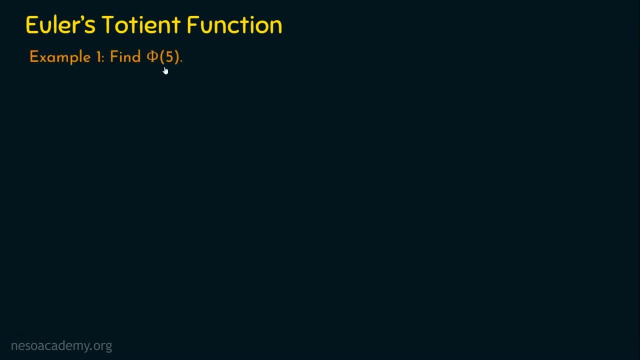 In the first example the question is: find phi of 5.. We have already solved this in the previous lecture, but in the previous lecture we did manually, isn't it? But see here how simply I'm calculating Here. n is equal to 5, because that is what is given in the question. Is n a prime? 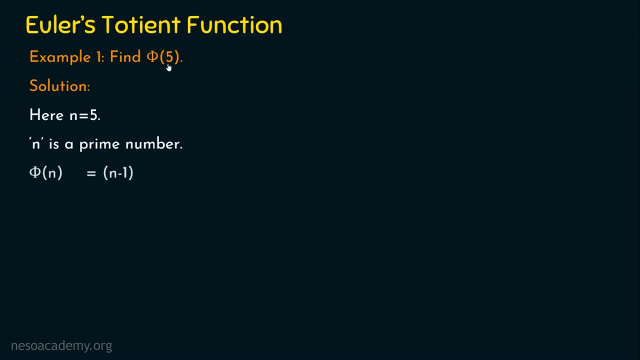 number. Yes, If n is a prime number, then what's the formula? we have seen Phi of n is equal to n minus 1.. So we have already solved this in the previous lecture. Now let's see how to solve. 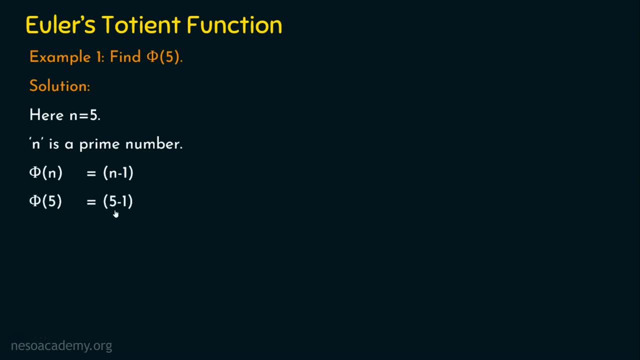 So we are going to compute phi of 5.. So phi of 5 is equal to 5 minus 1, which is equal to 4, and that's what the answer. So phi of 5 is equal to 4.. What do you mean by this? There are 4. 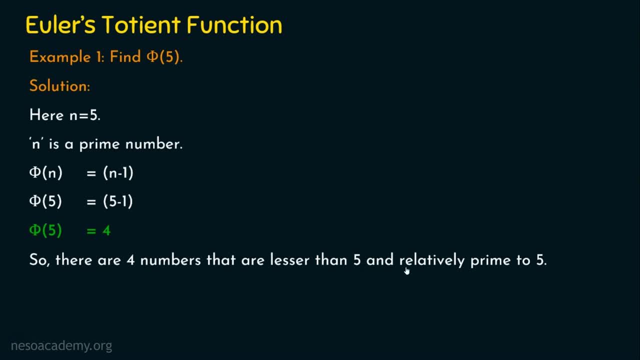 positive numbers that are less than 5, that are relatively prime to 5.. That is what this number 4 says. right, That is what this Euler's torsion function is all about. I think the example number 1 is clear to you. Let's see example number 2.. In example number 2, we are going to compute phi of 5. 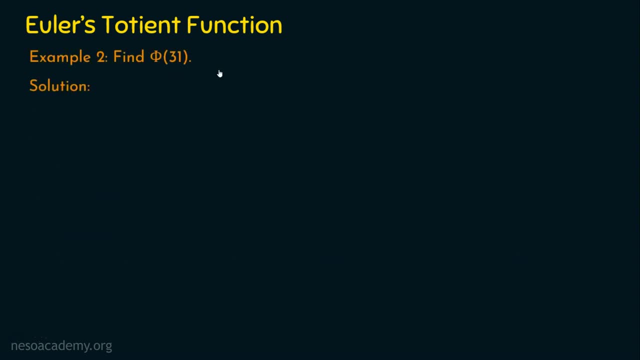 to find phi of 31.. So let's solve this. We know n is given as 31.. So obviously 31 is a prime number. So we can easily apply this: phi of n is equal to n minus 1.. So when you apply n value. 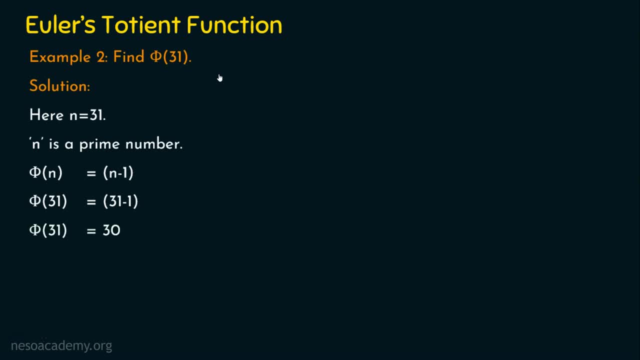 you get, phi of 31 is equal to 30. So the answer for this question is 30. So it means there are 30 positive integers that are lesser than 31 are relatively prime to 31.. The idea behind this is: 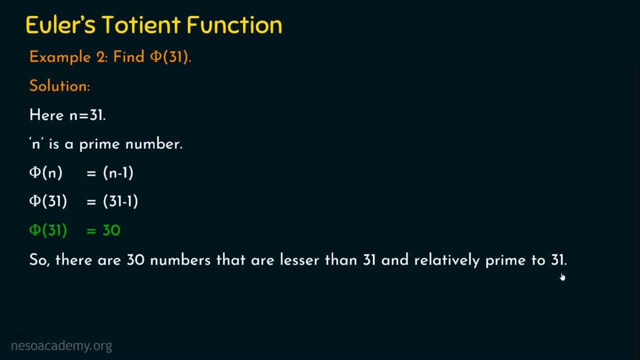 so simple. If n value is a prime number, we can easily compute phi of n, n minus 1.. But what if n is not a prime number? So let's see that kind of examples also. Let's step into example number 3.. In example number 3, we are going to compute phi of 35. So let's solve. 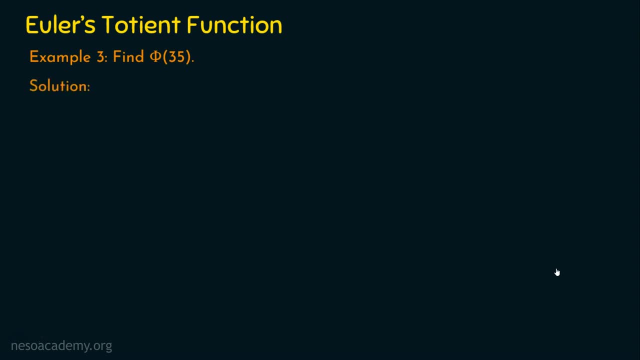 this now. Now we can clearly say that 35 is not a prime number, But 35 is a product of two different prime numbers, 5 and 7, right? So 35 can be factored into 5 and 7. So it is a product. 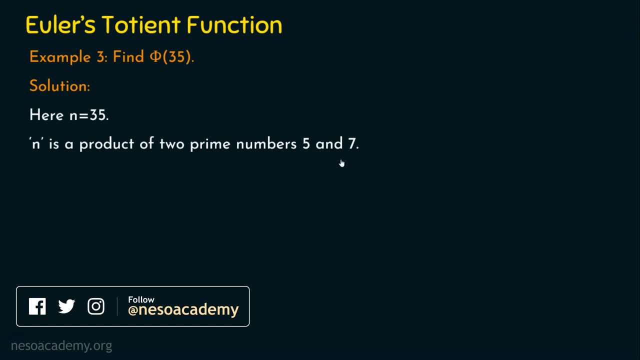 of 5 and 7, where 5 is a prime number. So let's see that kind of example. So let's see that kind of example. So 5 and 7 are different prime numbers. So let's assign p is equal to 5 and q is. 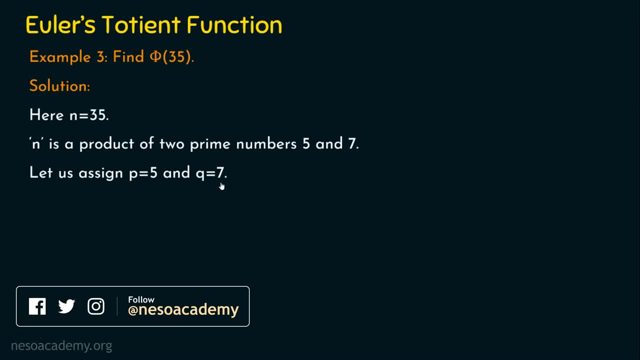 equal to 7.. You can assign p is equal to 7 and q is equal to 5 as well. No worries, both will give the same result, obviously. So we know the formula is: phi of n is equal to p minus 1 into q minus 1.. 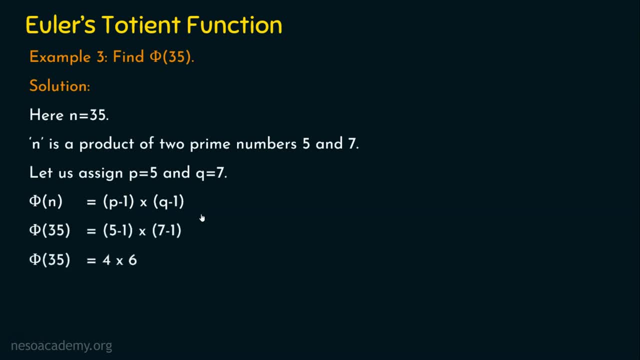 So when you solve this, you get 5 minus 1 into 7 minus 1, which is equal to 4, into 6, which is equal to 24.. So the answer is 24.. What do you mean by this? There are 24 numbers, So 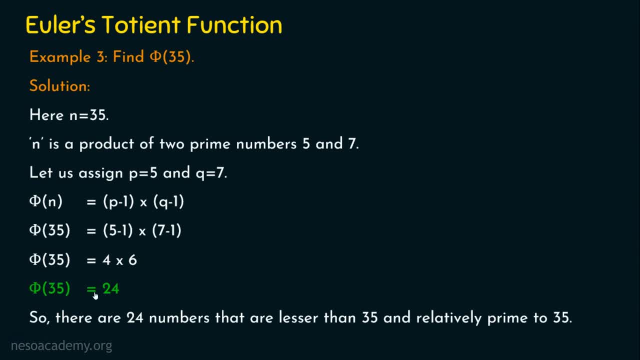 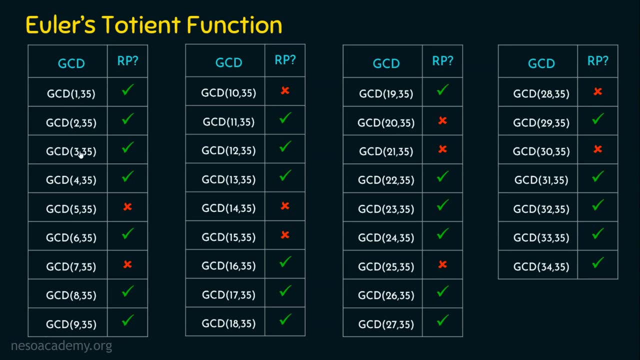 24 positive numbers, to be precise, that are less than 35 are relatively prime to 35. Just think, if there is no formula and you are asked to do it manually. Obviously you should have followed this approach right. So we are starting from gcd 1 comma 35, 2 comma 35, 3 comma 35, up to gcd. 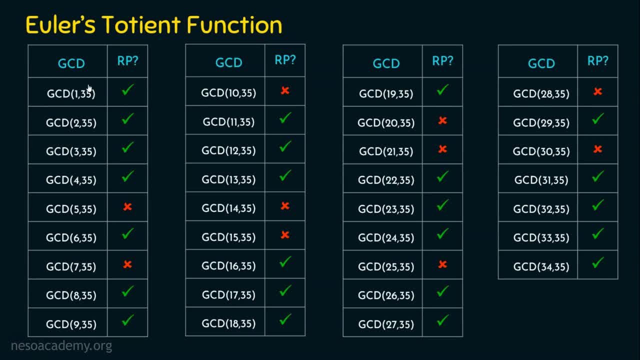 34 comma 35. And obviously we are going to compute whether they are relatively prime. If the remainder is 1, then obviously they are relatively prime, isn't it? So if you compute here, there are certain numbers that are relatively prime to each other. Say, 4 and 35 are. 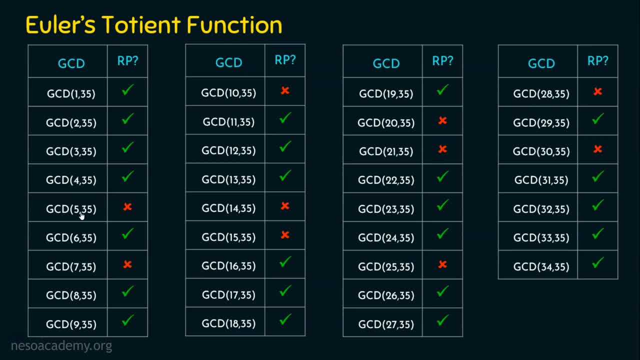 relatively prime to each other, because the gcd value will be 1.. But in this case these two are not relatively prime because 5 and 35 can be divided by 5, the greatest number right, The greatest common divisor. So here gcd of 5 comma 35 will be 5, and hence 5 and 35 are not relatively. 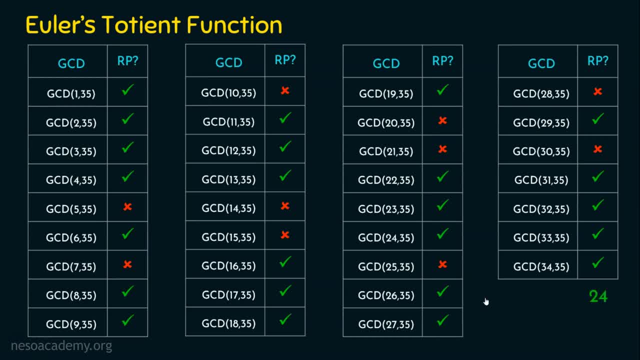 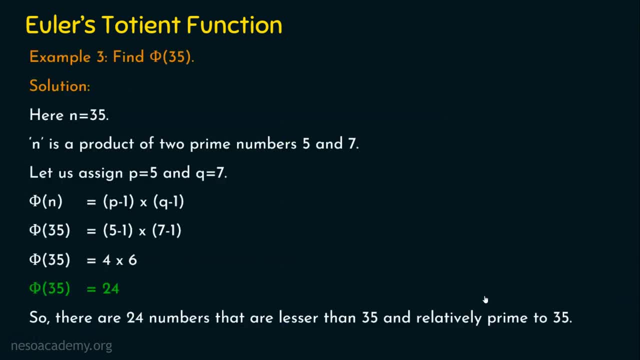 prime numbers. So if you manually do this, you will get 24 numbers that are relatively prime numbers. If you calculate, you will get 24.. But see how easily we did this here. It's so simple, because 35 is a product of two different. 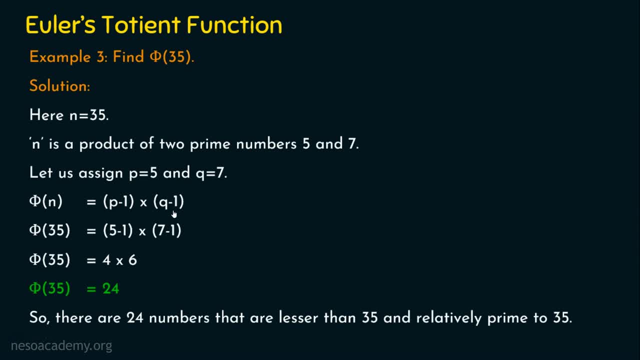 prime numbers. So we use the formula: 5 of n is equal to p minus 1 into q minus 1.. Now I wanted to give you an important instruction here. Let's say we are going to compute 5 of 25.. 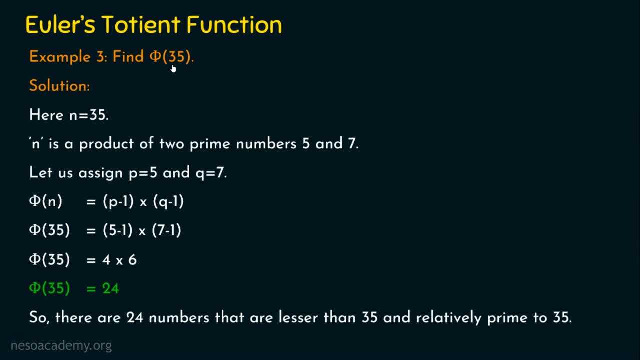 And if you are given with the question 5 of 25, so 5 of 25 can be written as the product of two prime numbers, 5 and 5, right, But remember when you are going to compute 5 of 25, you cannot apply. 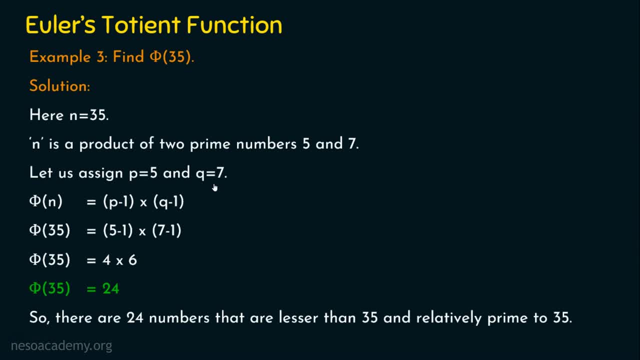 this formula? Why? Because p and q should be different. If you are going to compute 5 of 25, then p is equal to 5 and q is equal to 5, right? So this formula will never work out, in that. 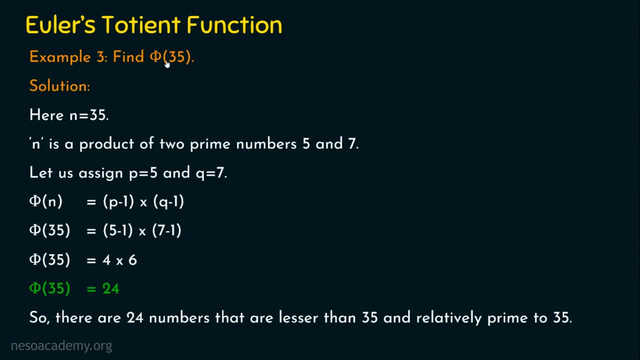 circumstance, And that's why I told you, if you are going to compute 5 of n, which is this, then it can be p minus 1 into q minus 1, only if p and q are different. I think things are clear. 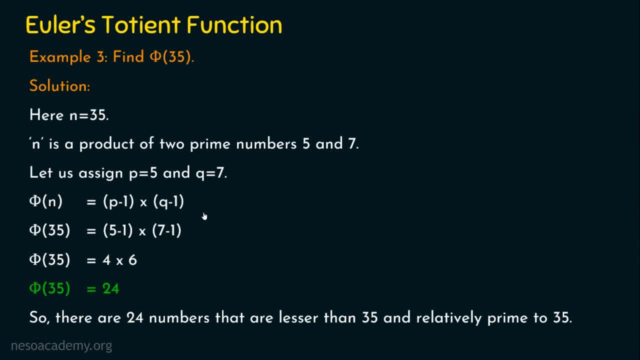 for you. Now you may be asking: if 5 of 25, we are given with how to compute For that, only the third formula. let's see some examples which are matching criteria number 3. Example number 4. The question is: find 5 of 1000.. I already told you in the last lecture that if you 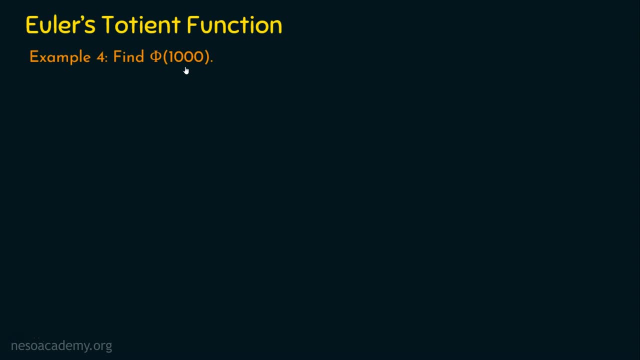 are asked to find 5 of 1000,. it is a time-consuming process if you manually do it, like gcd of 1, 1000, gcd of 2, 1000, up to gcd of 999, 1000.. At the same time, if this number 1000 can be a. 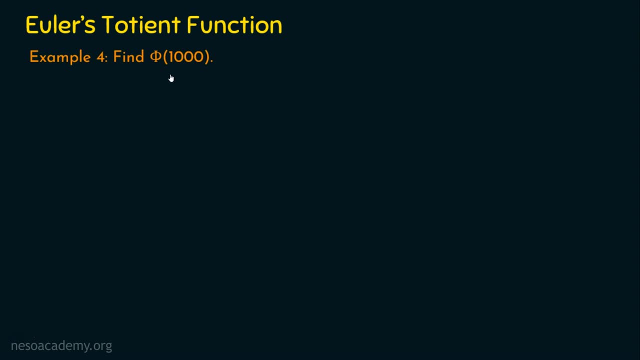 product of two different prime numbers exactly, then we can go for the first one, which is 5 of n is equal to p minus 1, into q minus 1.. But we can't expect all the numbers to be falling with criteria 1 or criteria 2.. There are chances for criteria 3 as well, isn't it, And that's why we. 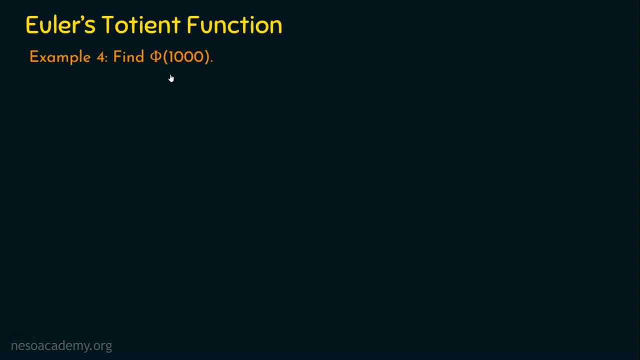 have landed up with example number 4.. And we are now seeing examples for criteria 3, which I had shown previously. Let's solve this now Here: n is equal to 1000.. If you factor this 1000,, you will. 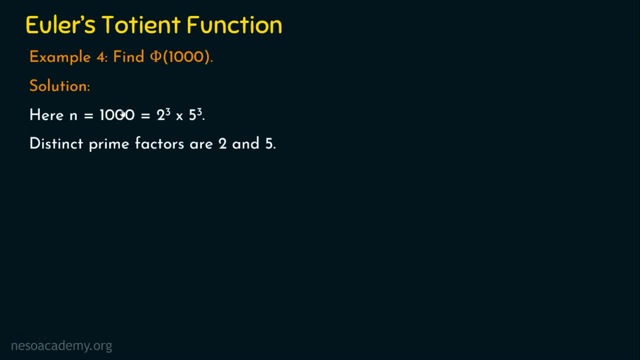 get 2 power 3 into 5 power 3. See, if you factor this, you may get 100 into 10, also 100 into 10, again, you factor When you factor to the core, as I already mentioned when I explained. 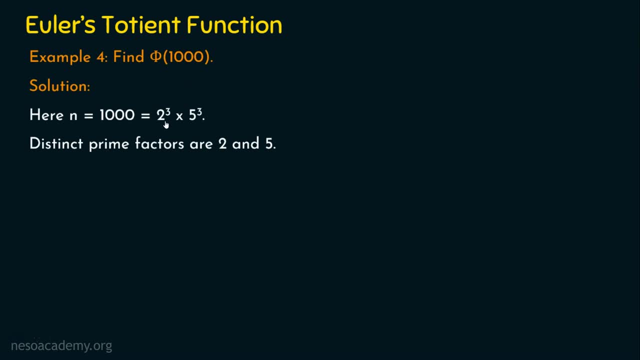 you about prime numbers, ultimately the base numbers will be prime numbers, right? So any number if you factor, ultimately the base number will be prime numbers. So 1000 can be 2 power 3 into 5 power 3.. So 2 power 3 is 8, 5 power 3 is 125.. 125 into 8 is obviously what 1000. This. 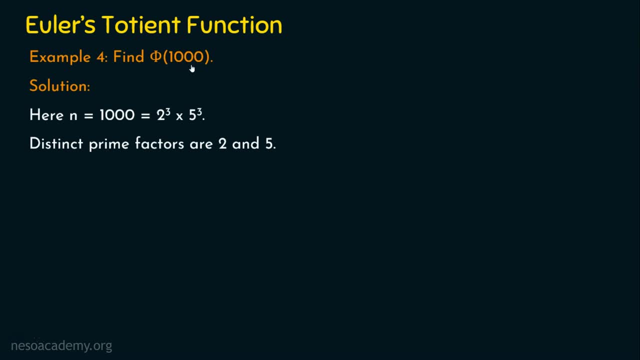 can be with any combo, right. So this can be 500 into 2 or 250 into 4, or 100 into 10, or 50 into 20.. But ultimately when you divide to the core, you will get prime factors. So we are factoring this like this. So how many distinct? 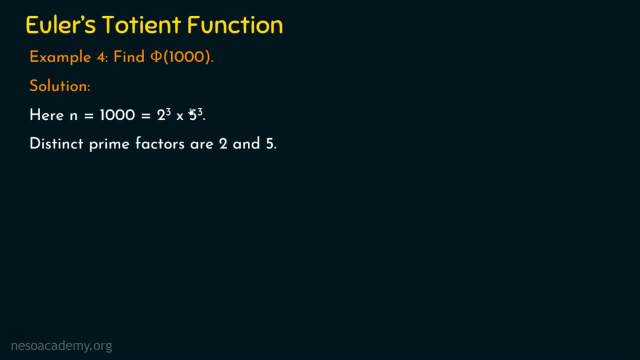 prime factors we have. One is 2 and the other one is 5. So we are getting distinct prime factors are 2 and 5. So here we have two different prime numbers. So we are taking the formula like this: 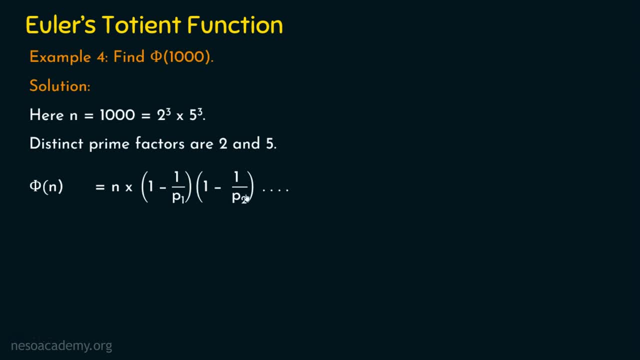 5 of n is equal to n into 1 minus 1 by p1, into 1 minus 1 by p2.. In case, if you are having other prime numbers, extend this as long as you have the number of prime numbers. Say, if you have two more prime numbers here, then you make it like 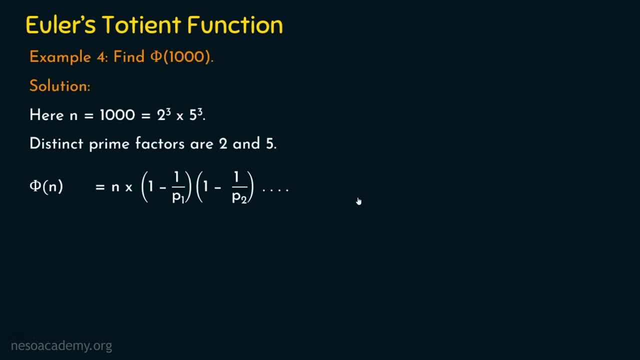 1 minus 1 by p3. Additionally, you just add it and 1 minus 1 by p4. Since we have only two distinct prime numbers, I am restricting this formula up to p2.. Now we know what is p1, right, Which is 2.. 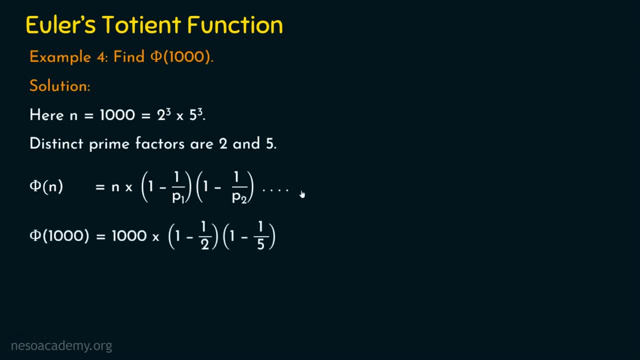 We know what is p2,, which is 5.. They are distinct prime numbers, So I am just substituting this and after evaluation I will be getting 5 of 1000 as 400. So the answer for this question is 400.. See how easily I solved this. It doesn't mean that. 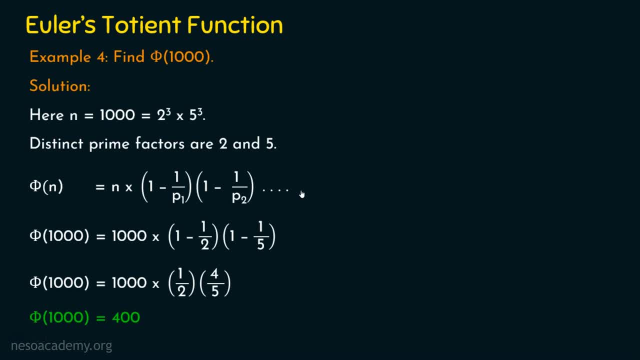 we cannot manually solve this, but think of if you go and do it manually It's obviously time consuming, but we got that. there are 400 positive integers that are less than 1000 are relatively prime to 1000. How easily we obtained this. Let's see one more example, Example number 5,. 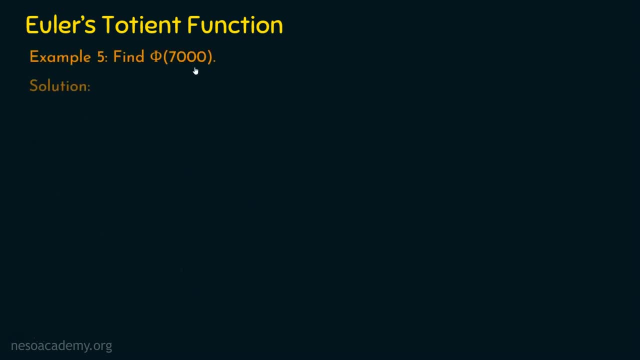 which is finding 5 of 7000.. So here n is given as 7000,, right? This 7000, can be written as 2 power 3 into 5, power 3 into 7 power 1.. So obviously we have distinct prime. 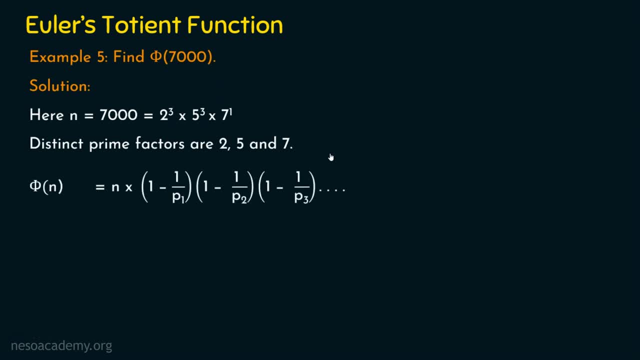 numbers as 2, 5 and 7.. You need to add one more prime number here in the formula, which is: 5 of n is equal to n into 1 minus 1 by p1, into 1 minus 1 by p2, into 1 minus 1 by p3. We have only three. 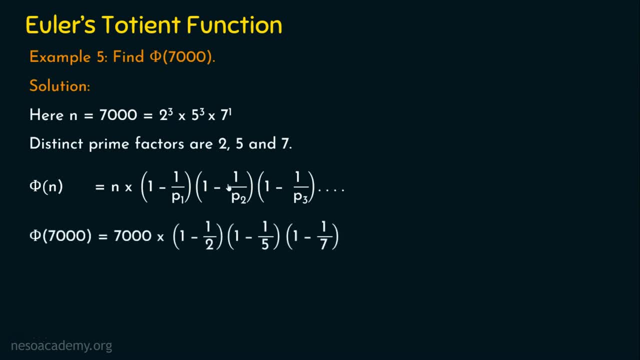 distinct prime numbers. Now let's solve this now. So when you apply p1 as 2, p2 as 5 and p3 as 7,, after simplification, we get the final result as 2400.. Final answer for this question is 2400.. It means there are 2400 positive integers that are less. 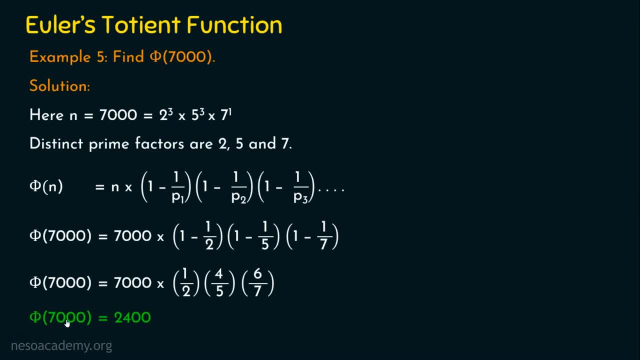 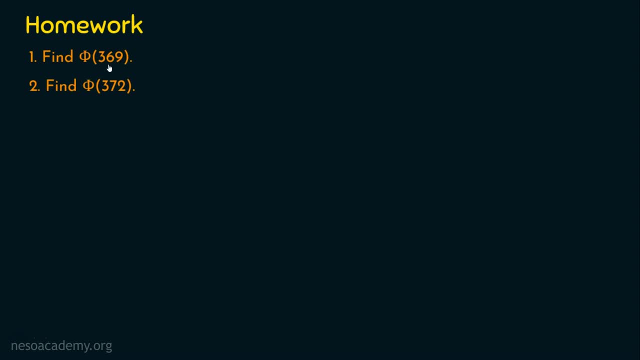 than 7000 that are relatively prime to 7000.. And that's it, guys. Before we step out, let's see the homework question. I have given two homework questions. You are required to find 5 of 369 and find 5 of 372.. After solving this, I request you to post your answers in the comment.